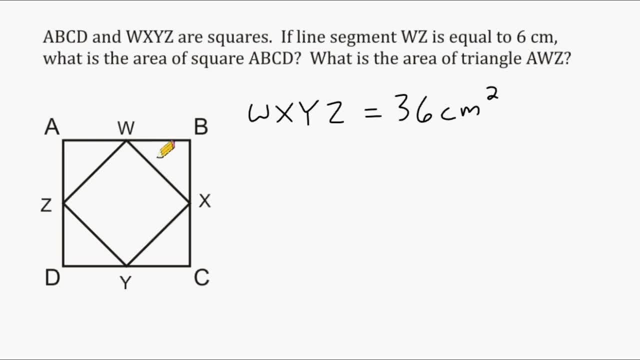 Because we have a 6 by 6 square. we just take 6 and multiply it by itself or square it. Now the problem did not ask us to figure out the area of WXYZ, but we need to know this information Because what we're going to do next is we're going to take this square. 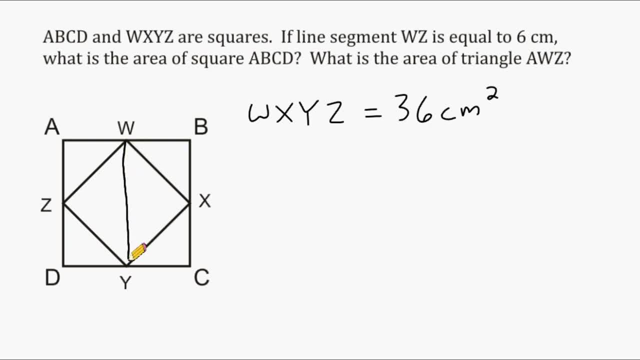 here in the middle, and we're going to divide it into four equal parts. Now, by doing this, what we did is we took the entire figure and created 1,, 2,, 3,, 4,, 5,, 6,, 7,, 8,, 9,, 10,, 11,, 12,. 13,, 14,, 15,, 16,, 17,, 18,, 19,, 20,, 21,, 22,, 23,, 24,, 25,, 26,, 27,, 28,, 29,, 30,, 31,, 32,, 34,, 35,. 35,, 36,, 37,, 38,, 39,, 40.. Now what we're going to do next is we're going to take the whole area of WXYZ and divide it into four equal parts, So it's going to be 4,, 4,, 6,. 7,, 8,, 9,, 10,, 11,, 11,, 12,, 13,, 14,, 14,, 15,, 18,, 19,, 20,, 21,, 23,, 24,, 35,, 36,, 37,, 38,, 39,, 40. 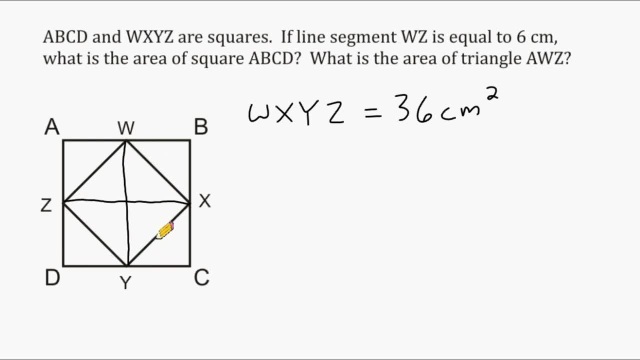 Now we know if this center square here is 36 square centimeters and we divide that into four equal parts, that means that each one of these four triangles must be equal to 9 square centimeters, And because these four triangles are identical to these four, 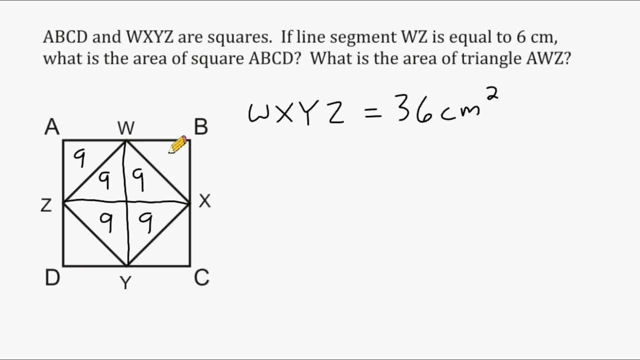 triangles. Each one of those are also an area of 9 square centimeters. So, basically, we created 8 identical triangles, each with an area of 9 square centimeters. So all we have to do is take 8 and multiply it by 9 to get a total of. 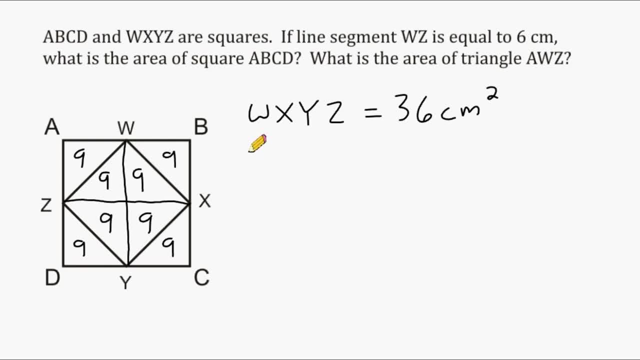 72 square centimeters. So we can say that square ABCD is equal to 72 square centimeters. And we also have to make a statement about the area of triangle AWZ, which is this right triangle right here, which is equal to 9 square centimeters. 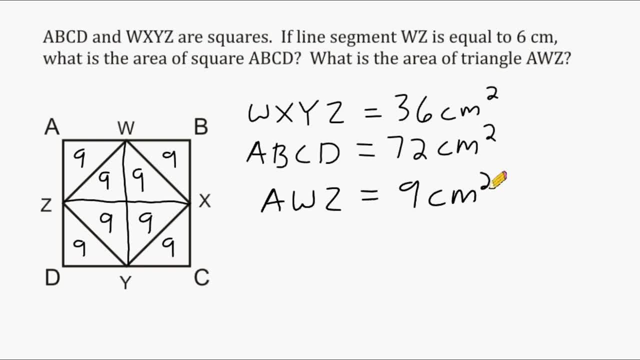 So really the key to this problem was to divide this diagram into all congruent triangles. But we really had to know that this middle square here had an area of 36 square centimeters. first, by knowing that this line segment right here is a length of 6 square centimeters, And if this line 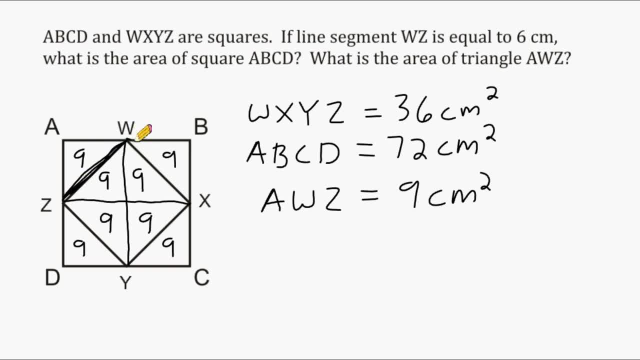 is 6, that means that this side of the square is 6, and a 6 by 6 square would result in an area of 36.. And then, by dividing this into four equal parts, we can figure out that each one of these four triangles has an area of 9 square.